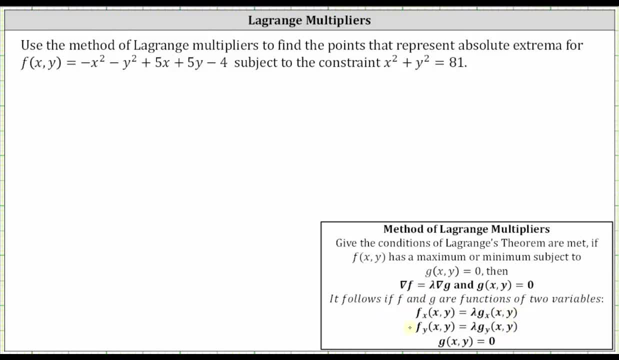 we need to solve the system of equations shown here below, involving the partial derivatives as well as the constraint, in the form of g of x comma y equals zero. So we have f of x comma y, but we need to write the constraint: x squared plus y squared equals 81. 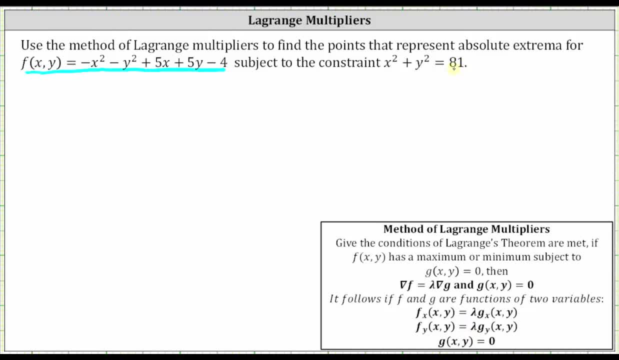 in the form of g of x comma y. To do this, we need to set one side of the equation equal to zero. Let's go ahead and subtract 81 on both sides, which gives us g of x comma y equals x squared plus y squared minus 81.. 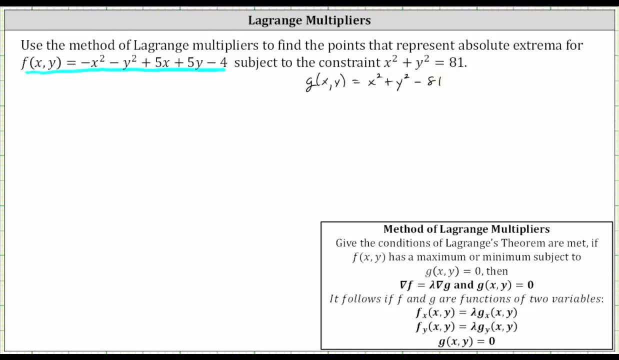 And now let's work on setting up the first equation given by the partial of f with respect to x equals lambda times the partial of g with respect to x. So for the partial of f with respect to x, we differentiate f with respect to x. 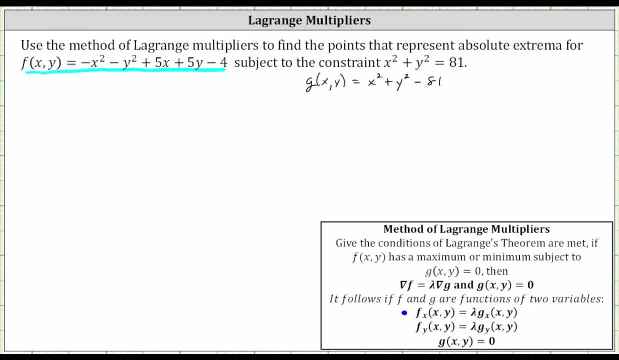 treating y as a constant, which gives us negative. two x plus five equals lambda times the partial of g with respect to x, which is equal to two x. For the second equation we have: the partial of f with respect to y equals lambda times the partial of g with respect to y. 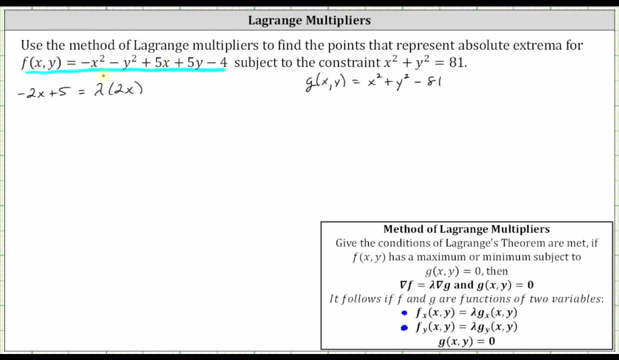 For the partial of f with respect to y. We differentiate with respect to y, treating x as a constant, which gives us negative. two y plus five equals lambda times a partial of g with respect to y, which is two y. And our third equation is: g of x comma y. 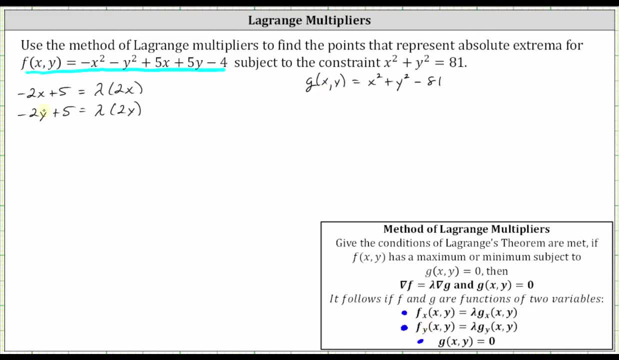 equals zero, which is x squared plus y squared minus 81 equals zero. And now to begin to solve the system of equations, we will solve the first equation for x and the second equation for y. To solve the first equation for x, we need to get the terms with the factor of x. 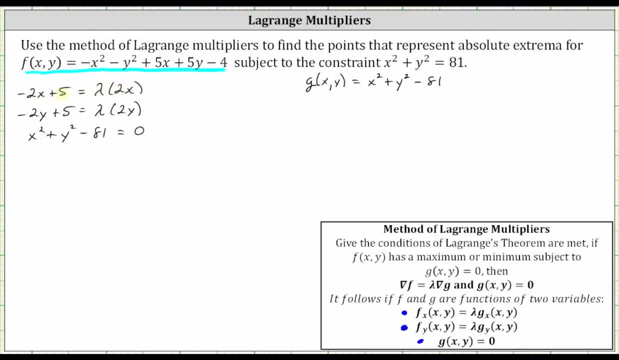 on the same side. Let's go ahead and add two x to both sides and also change the order of the equation. Let's write the equation as: two x lambda plus two x equals five. Next, factor out two x, giving us with two x times the quantity. 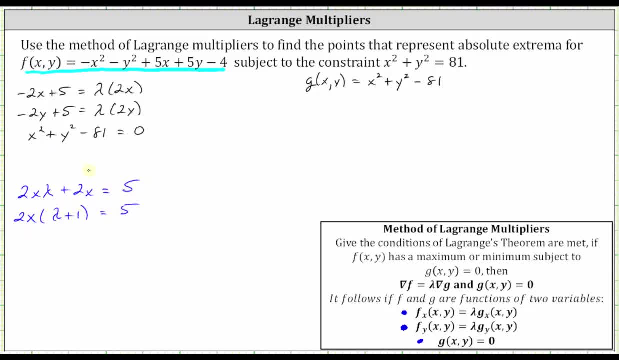 lambda plus one equals five. Next, we divide both sides of the equation by lambda plus one. Simplifying, we have two x equals five divided by the quantity lambda plus one. Instead of dividing both sides by two, let's multiply both sides by one half. 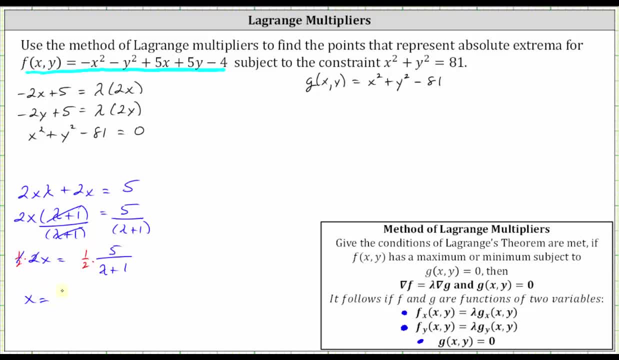 Simplifying: we have x equals. let's write the right side as five divided by the quantity two lambda plus two. And now we need to solve the second equation for y, and we'll follow the same procedure. We will add two y to both sides. 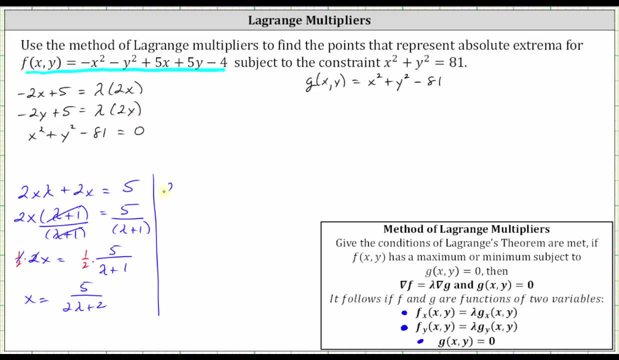 and change the order of the equation. We have two y lambda plus two y equals five. Factor out two y, Divide both sides by lambda plus one, which gives us two y equals five divided by the quantity lambda plus one, And once again solve for y. 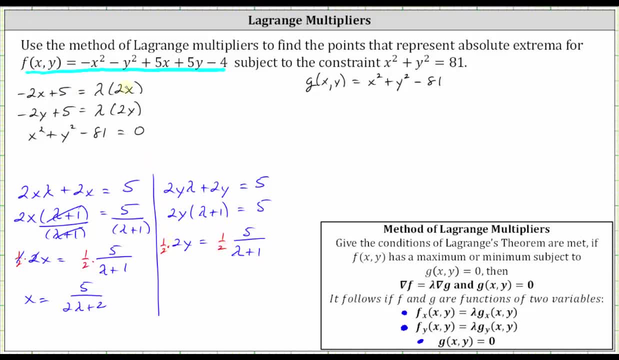 we will multiply both sides by one half Simplifying, we have: y equals five divided by the quantity- again two lambda plus two. So what's special about this is notice how both x and y are equal to five divided by the quantity. two lambda plus two. 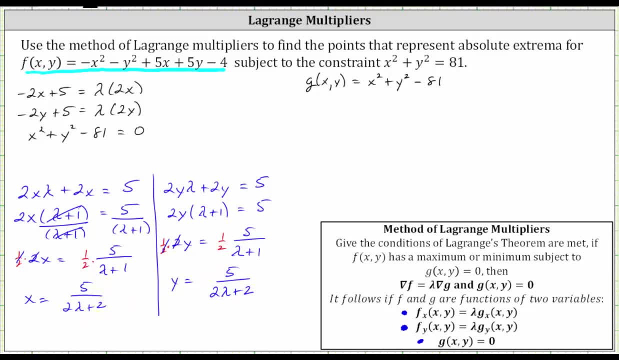 So what's special about this is notice how both x and y are equal to five divided by the quantity two lambda plus two. So the important thing that we just discovered for these first two equations is we now know x is equal to y. Knowing this, we can now substitute x for y. 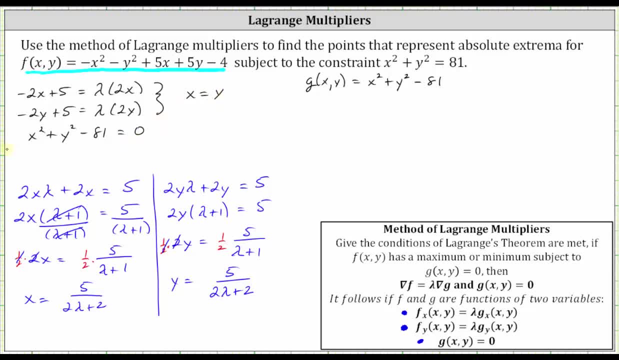 or y for x in the third equation and then solve for the single variable. Let's go ahead and substitute x for y. Performing the substitution gives us x squared plus x squared. Let's also add 81 to both sides equals 81.. 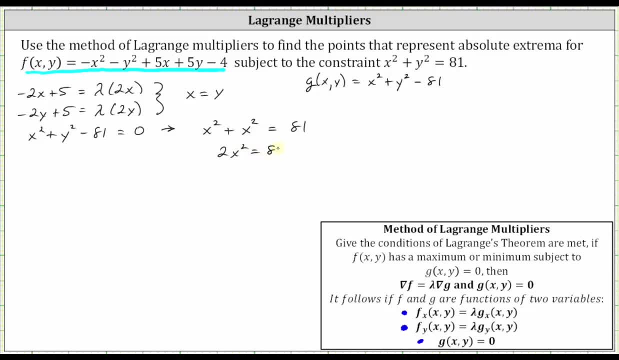 Combining like terms, we have two: x squared equals 81.. Divide both sides by two, Simplifying we have: x squared is equal to 81 halves. Take the square root of both sides. We are going to have a plus or minus value for x. 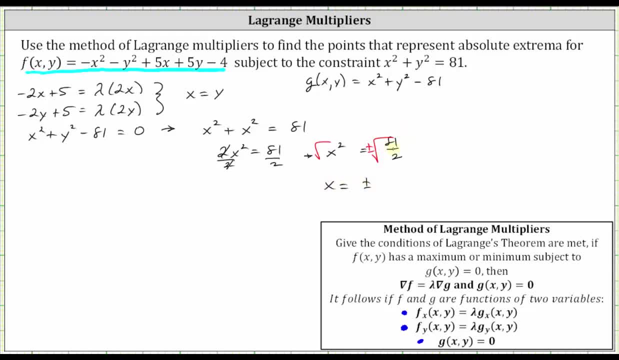 We now know x is equal to plus or minus. The square root of 81 is nine and we have the square root of two in the denominator. And remember x is equal to y, so we also know y is equal to plus or minus nine. 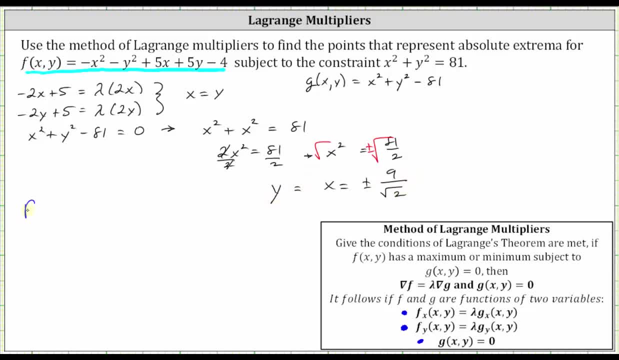 square root two. So we have two points to consider: One point where both x and y are positive- nine divided by square root two- And the second point where both x and y are negative. And now to find the z coordinates. 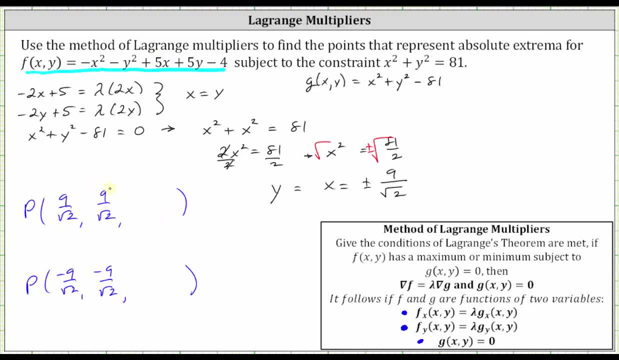 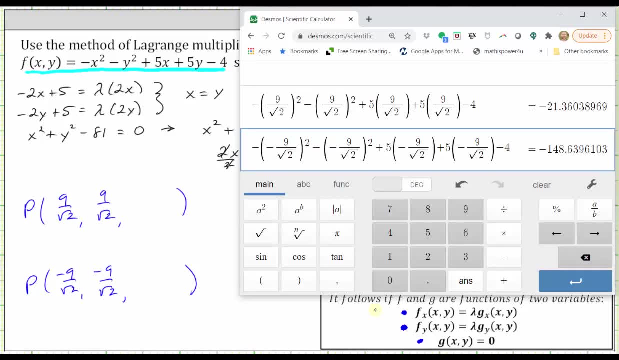 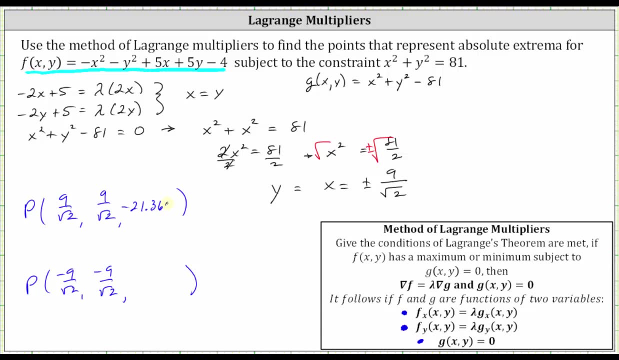 we need to evaluate the function f of x comma y, And I've already done this to save some time. Notice, when both x and y are positive, the function value is approximately negative: 21.3604.. And when both x and y are negative, 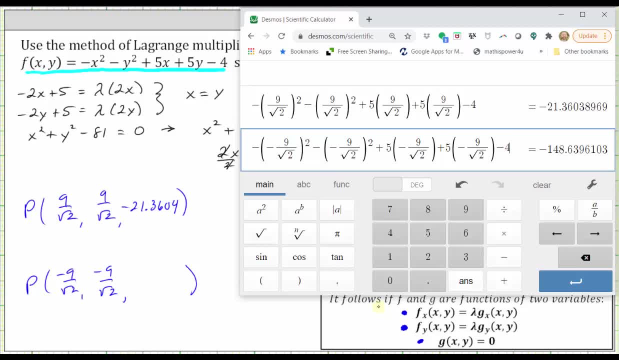 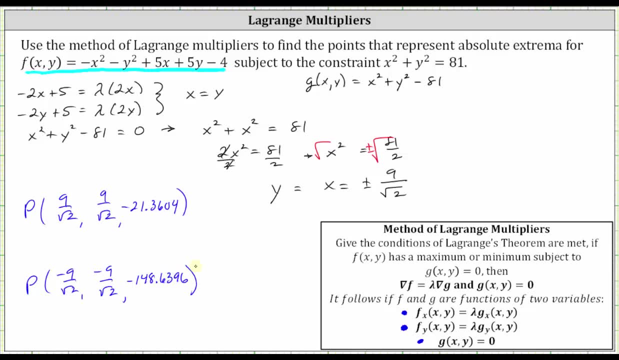 the function value is approximately negative: 148.6396.. So the largest function value represents the absolute maximum. The least function value represents the absolute minimum. So the absolute minimum is approximately negative, 148.6396.. The location is often given using the x and y coordinates. 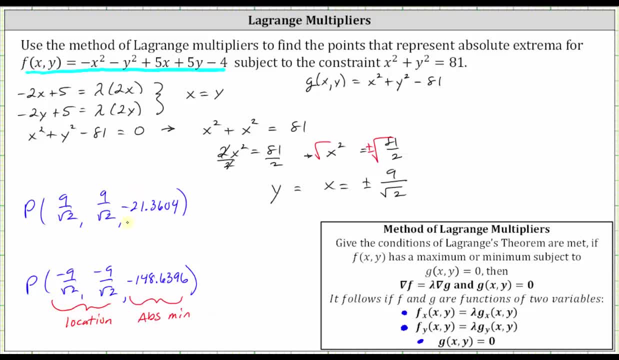 And the greatest function value or z coordinate is the absolute max. The absolute max is approximately negative 21.3604.. And the location is often given using the x and y coordinates, So it just depends on the question You may be asked to give. the order triples. 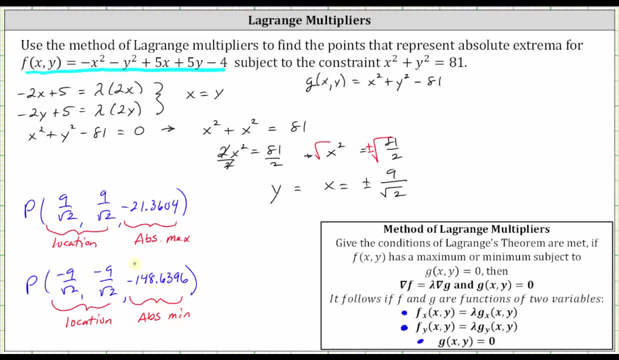 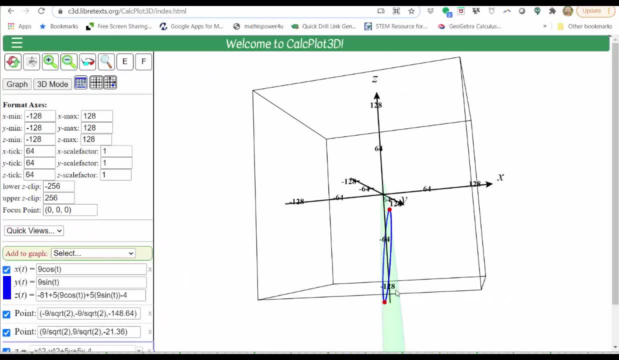 You may be asked to give the absolute max and min and their locations. Before we go, let's verify this graphically. The graph of f, of x, comma y is the graph of the green surface. This blue space curve is where the constraint intersects the surface. 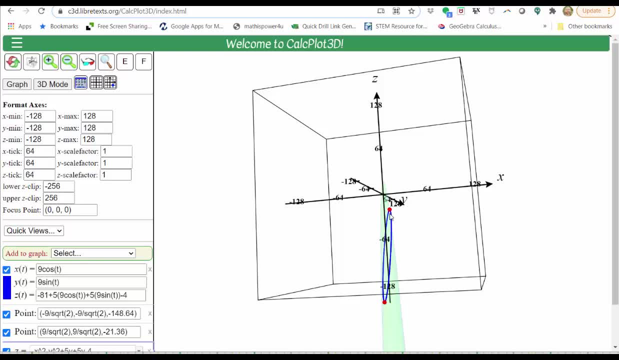 Notice how this red point here is the highest point that is on the surface and satisfies the constraint. This point represents the absolute max that we found. This point represents the absolute max that we found. This point represents the absolute max that we found And this low point is the lowest point. 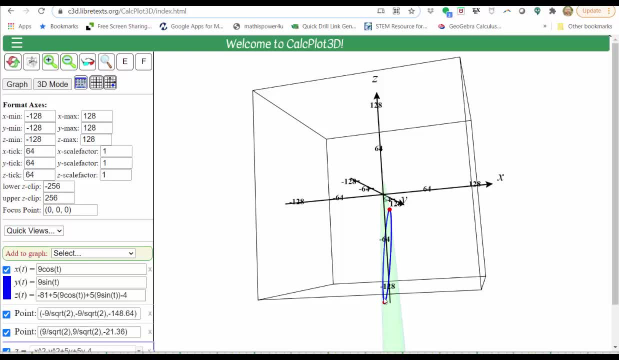 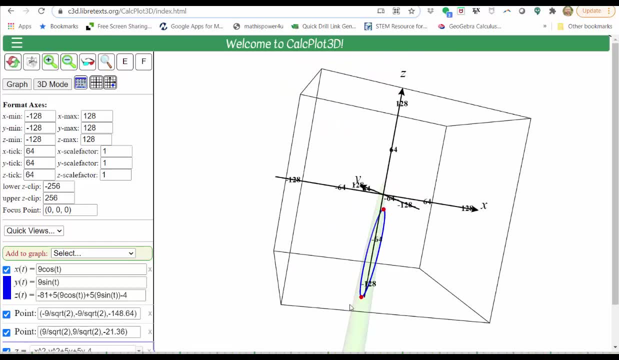 that also satisfies the constraint and is on the surface. This point represents the absolute minimum, So this graph does verify that our work is correct. I hope you found this helpful.